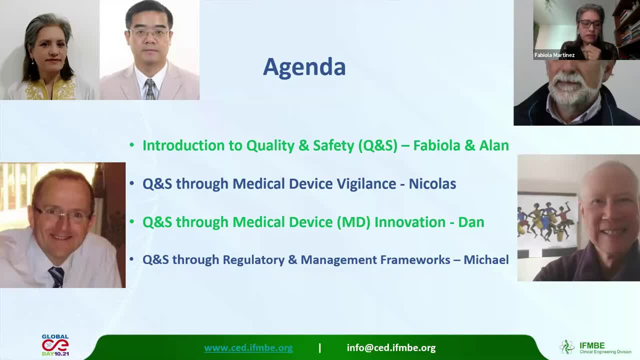 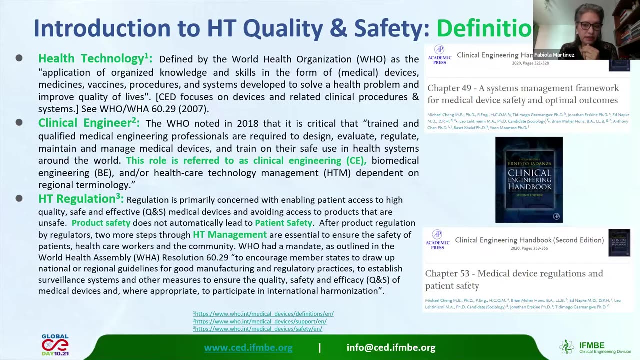 regulation and frameworks. Then we will have some minutes for questions from the audience. For this you can use the Q&A Next slide, please. Quality and safety in health technology is an essential topic in health care, since they have an intense influence on the outcomes of the several procedures on the patients. 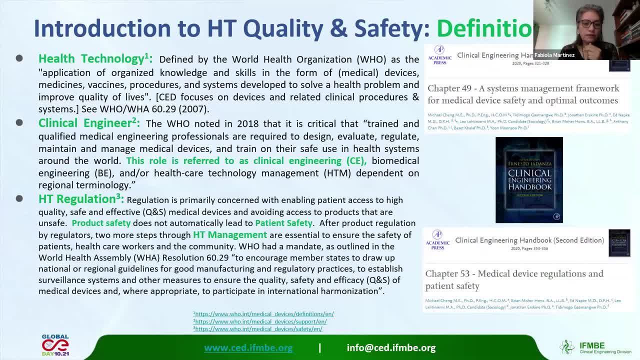 and also on the staff performance. So we made use of the definitions of health technology, clinical engineering and health technology regulation. In particular, this class concept emphasizes the importance of guaranteeing patient safety. We also have strong support on very valuable resources as a clinical engineering handbook. 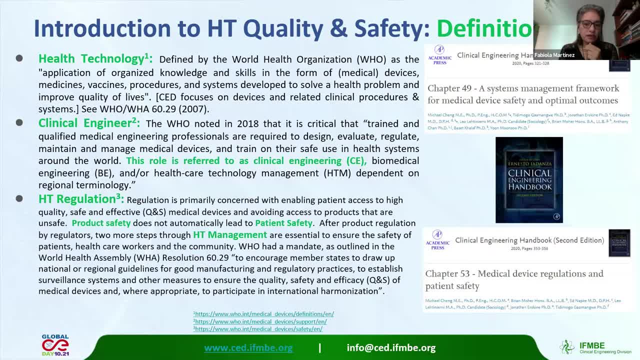 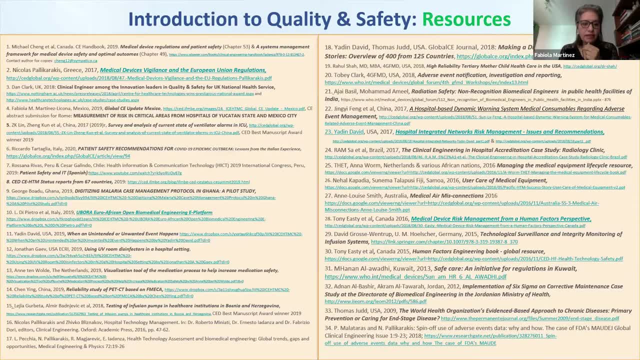 which chapters dealing with topics such as regulation and patient and medical device safety. Next slide, please. In addition to the clinical engineering handbook, other sources represent and other view of the aspects related to quality and safety in health technologies, from papers presented in international forums to public opinion, Including specific data on health safety. clinical engineering, health care and health, health research in particular. The Q&A is prepared. This slide shows that health care and health safety is a key aspect of this webinar, and not only the Q&A, but also the Q&A- health care and health technologies in general In particular. 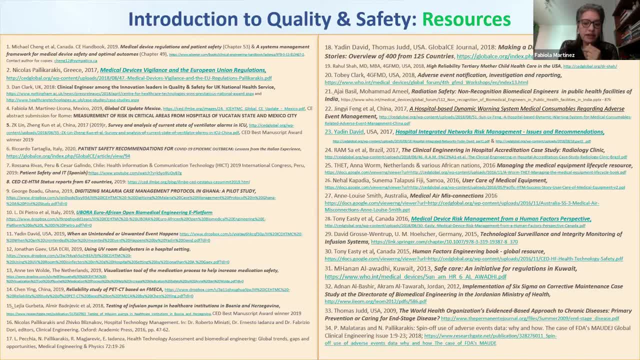 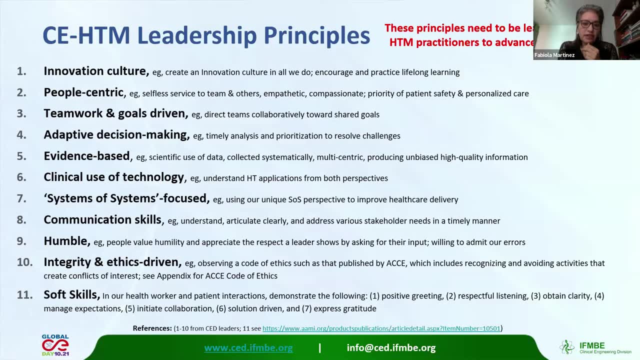 health care and health research in particular. In particular, health care and health research, in particular, publications with high impact in the clinical and HDA fields. Next, The functions of clinical engineers and health technology managers in quality and safety are governed by the principles of leadership that are presented. 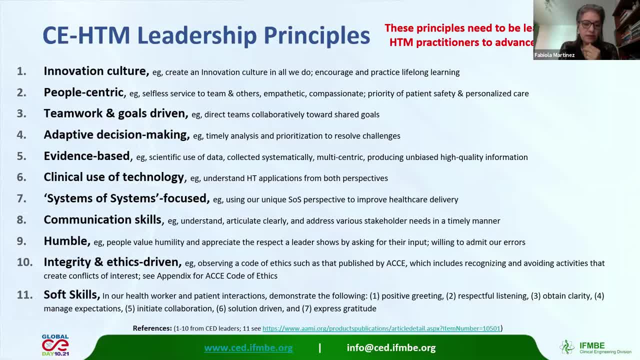 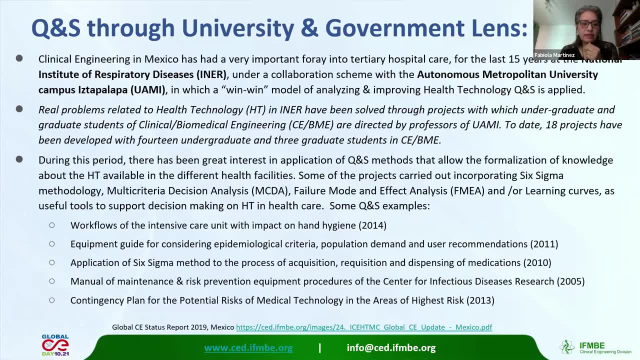 These principles need to be learned by all practitioners to advance their careers. Next, Academy and government can work together to achieve satisfactory levels of quality and safety in health institutions. The case I present is a 15-year collaboration where the university and a national health institute 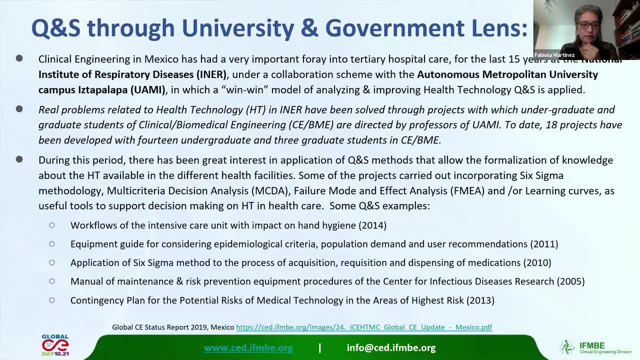 join forces to offer solutions to the various aspects of safety and quality that arise in the hospital environment. The way to develop this collaboration was through co-directed projects where the strengths of all parties were used, The university contributing with the professor's experience in research and methodological. 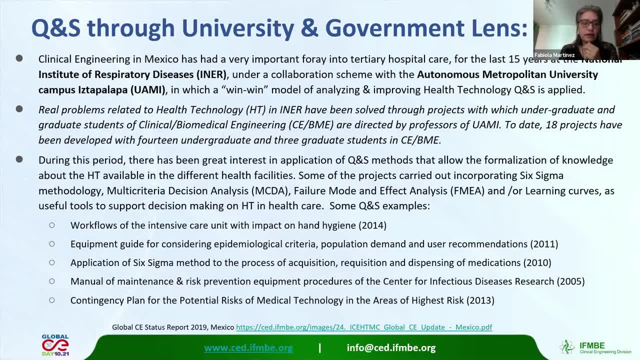 development And the institute contributing with the biomedical engineering department, expertise and domain of the clinical field, In this case a professor at the Universidad Autonoma Metropolitana and the heads of the biomedical engineering department of the National Institute of Respiratory. 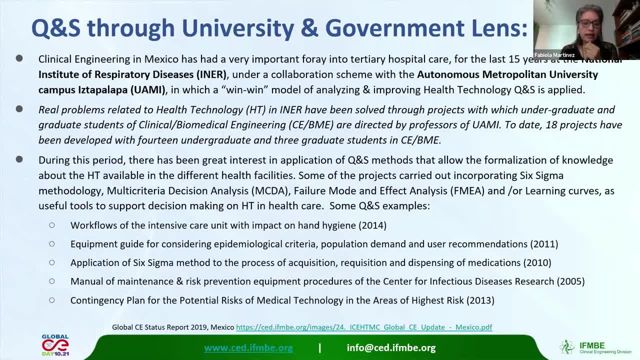 Diseases developed. undergraduate and graduate projects where the students proposed and implemented solutions to health technology associated problems. The experience gained in applying quality and safety methods and tools used in the research in other fields, allowing to deepen and generate knowledge that can be extrapolated to other health facilities. 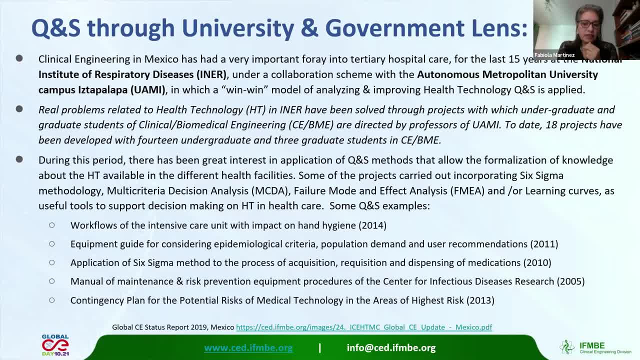 The sample of projects listed show the various aspects that can be addressed from the perspective of quality and safety. This scheme has been very positive for both parties, since they all involved obtain benefits. Most importantly, high value elements are provided for the safety of the patient. 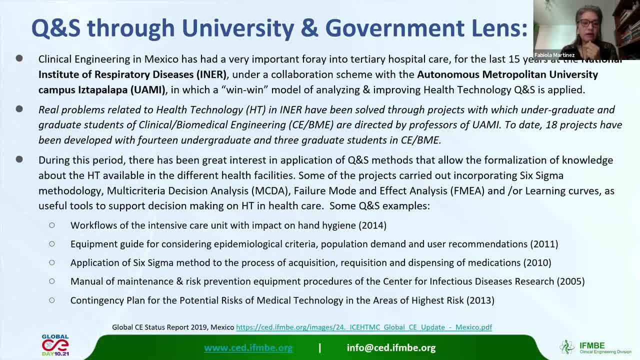 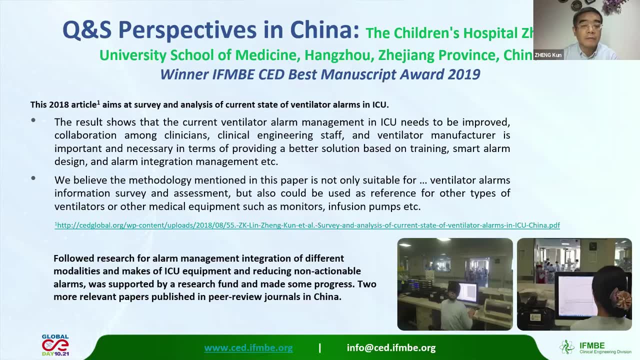 and the medical staff as well, for the quality of the functions in the institution. Now I welcome, Alan. Please go ahead. Thank you, Fabiola. Next slide, please. Hi everyone. Welcome to attend today's webinar at this special time. 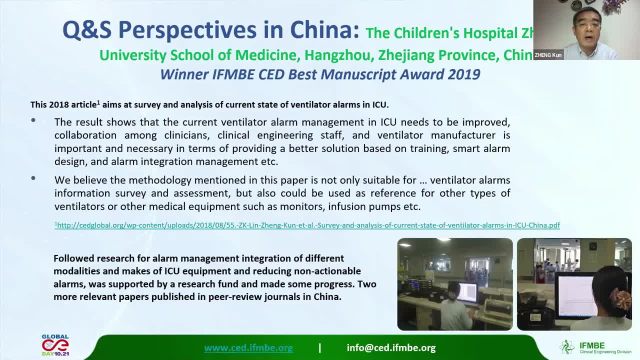 during the COVID-19 pandemic. Among all the routine tasks of hospital clinical engineering, service quality and safety is a cornerstone and an endemic. This is an internal topic which is the main theme of today's webinar. I'm Zeng Kun, director of logistic service department. 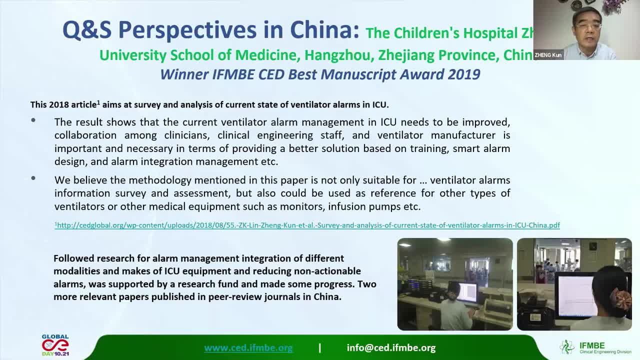 which includes clinical engineering and facility engineering. at the Children's Hospital of the Chang University School of Medicine in Hangzhou, China, My team is doing some projects aiming at improving quality and safety of technology for patient care. For example, as a slide shows: as a winner. 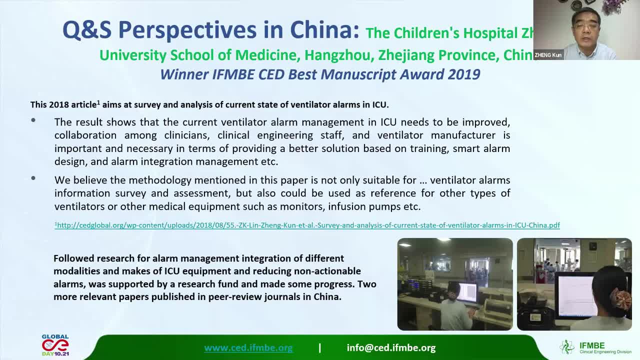 of IFMB-CED Best Manuscript Award 2019,. the paper addressed alarm management project in my facility. Based on the survey and analysis of medical equipment and alarm situation in ICUs at the hospital, several measures to reduce non-actionable alarms and address alarm fatigue are implemented.